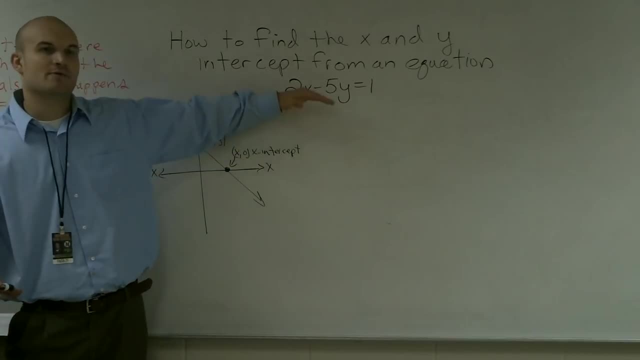 to learn later how to graph this equation, But there's a very simple way. we can also do this algebraically. that will help us find the x and y intercepts and then also learn how to graph it later. So the one key, important thing that I want to take from this graph is we notice that when the y intercept at 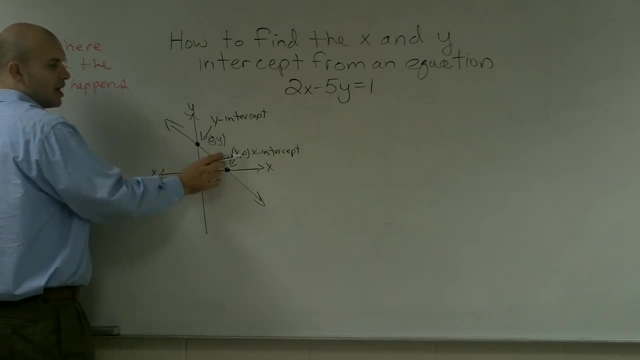 the y intercept x is 0. And at the x intercept our y value is 0. Because, remember, a coordinate point is x comma y. So here x equals 0. And at the x intercept y equals 0. So I'm 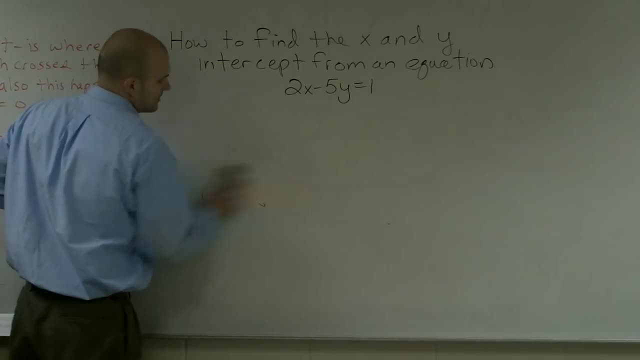 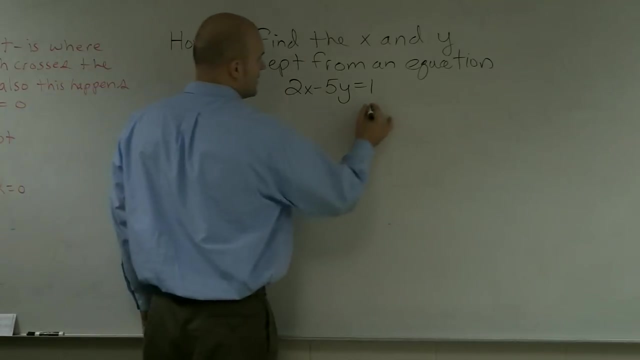 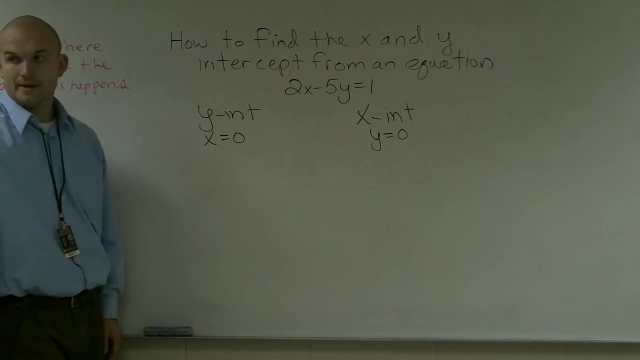 going to go ahead and erase this and then write those two different coordinates Properties. So at the y intercept x is equal 0. And at the x intercept y is equal 0.. OK, So what does it mean when one value is equal to 0? Well, what we can do is we can treat. 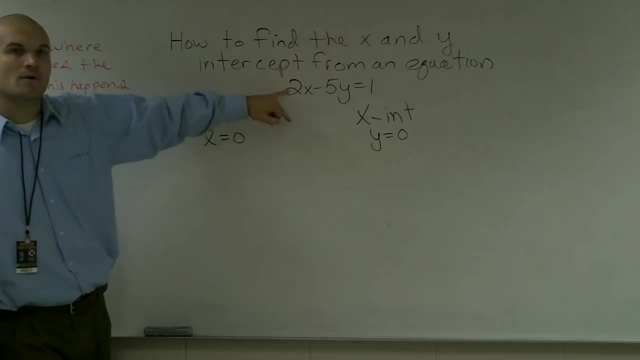 this as a function. And if we say 0,, x is now equal 0,. I'm going to now evaluate this for when x is equal to 0. So I'm going to plug in 2.. And I'm going to plug in 2.. And 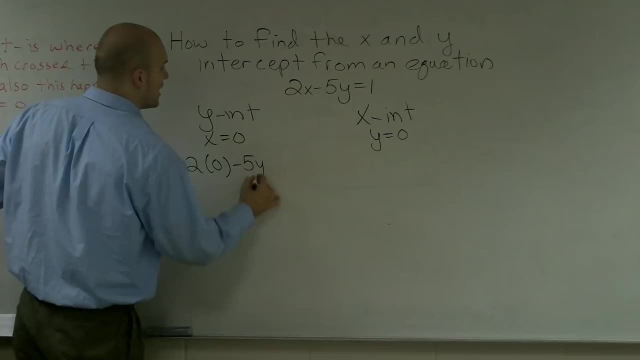 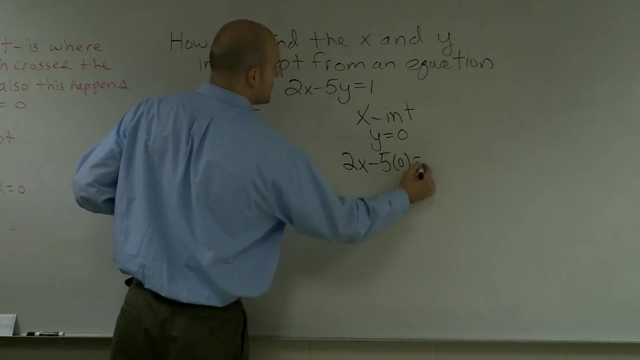 I'm going to say 2 times 0 minus 5 times y equals 1.. And then, over here, I'm going to say 2x minus 5 times 0 equals 1.. So now, looking at these two equations, now what I'm going. 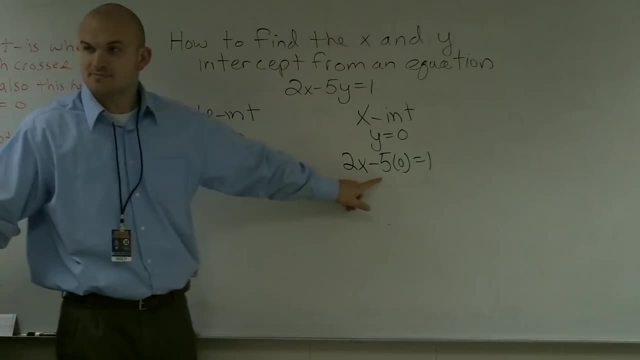 to do is for this one I'm going to solve for my variable y, And for this problem I'm going to solve for my variable x. So I know that anything multiplied by 0 is 0. So I'm just going to kind of cancel them out. So, therefore, I'm left with negative 5y And 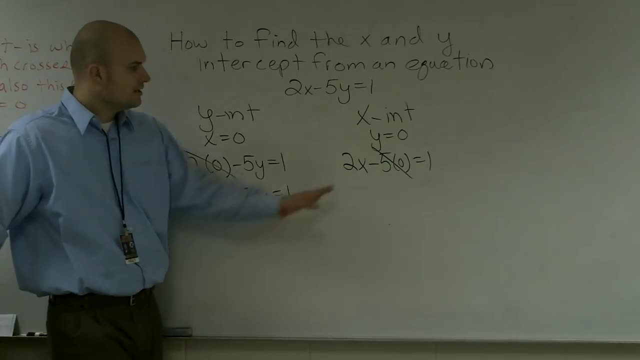 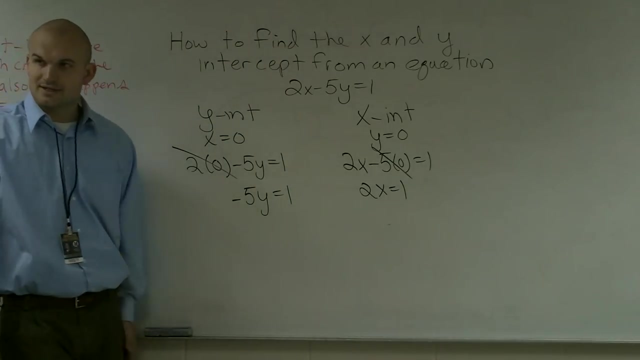 if I do this, I'm going to find the derivative of y equals 1.. And over here we have 2x equals 1.. So now we're just going to go ahead and simply go ahead and use our division-property of equality And since my negative 5 is multiplied by my y, I'm going to divide by negative 5. 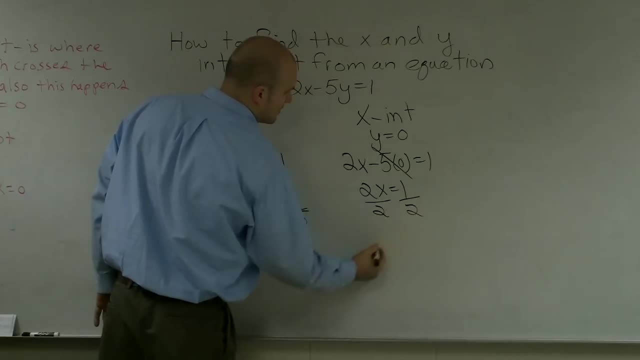 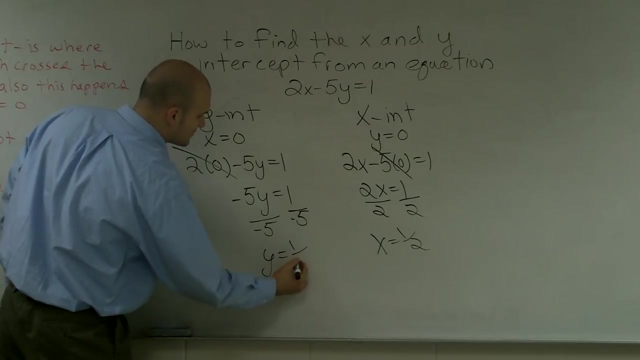 on both sides, And here I'm going to divide by 2 on both sides. Therefore x equals 1 half And here y equals a negative 1.. So what we can do, we can do a derivative of So, when going ahead and graphing my two points, if I know that, here's my y intercept, I know. 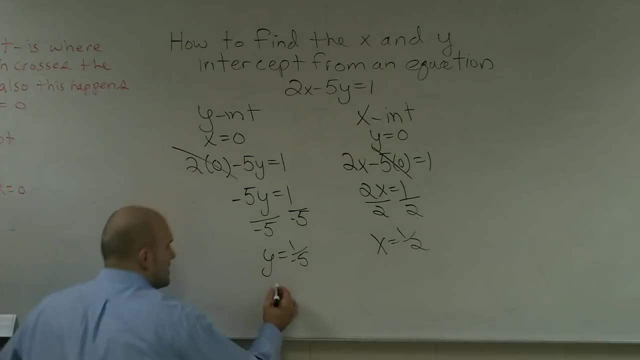 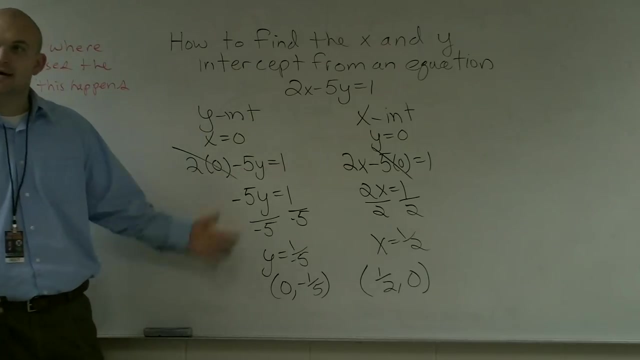 that x is 0 and my y value is negative 1 5th. my point is 0 and negative 1 5th and my point here is going to be 1 half 0.. So I can go ahead and plot these two points and they would be the two intercepts on my. 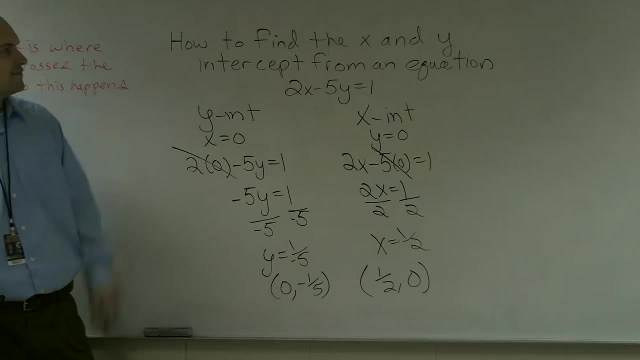 equation. Alright, so that's how you find the x and y intercept from an equation. 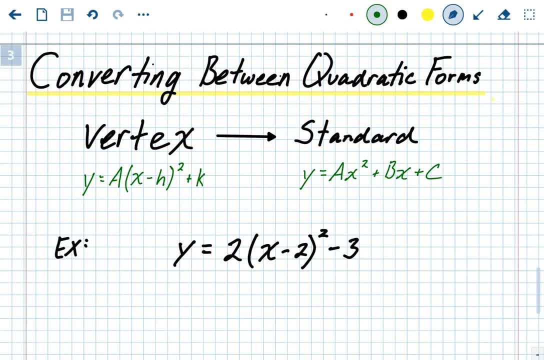 Okay, converting between quadratic forms, This one's got vertex form into standard form. Vertex form: y equals a times x minus h squared plus k, where h and k are your vertex Standard form. y equals ax squared plus bx plus c. c is your y-intercept. 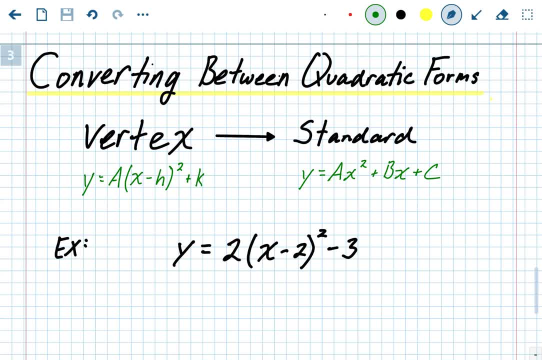 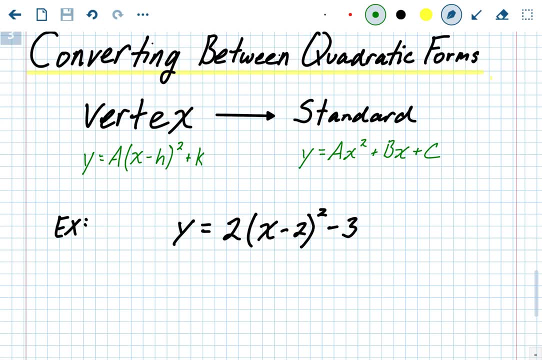 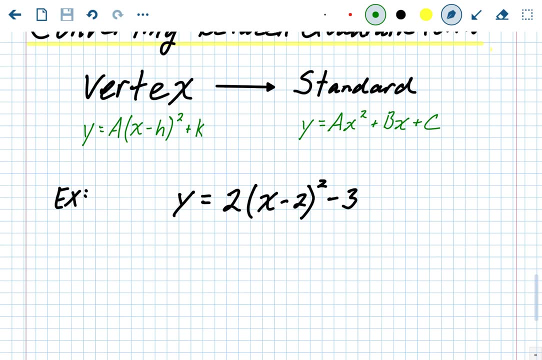 Again, each of these forms have something that you can find right away without doing any work. All right, so going vertex form into standard form is just basically going to be the same four steps each time. So in this problem we have y equals 2 times x minus 2, squared minus 3.. 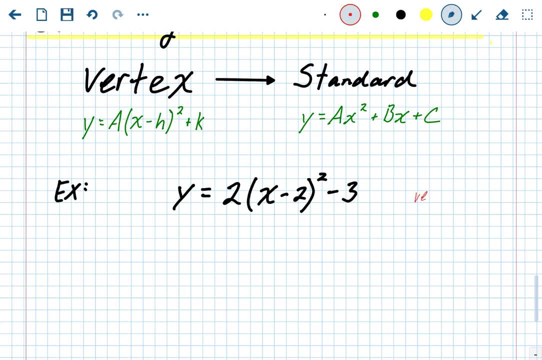 Again, I always like to just you know, write down what I know. If we're in vertex form, we know what the vertex is. The vertex in this one is the opposite of the inside and the outside. So it's going to be positive 2, negative 3.. 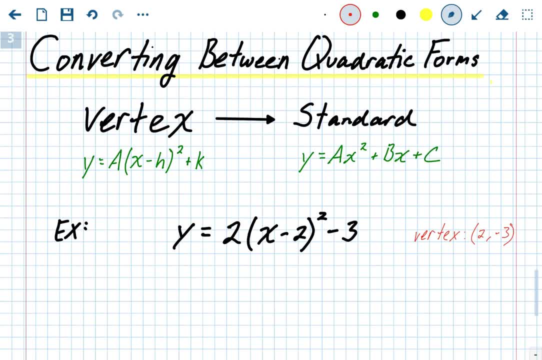 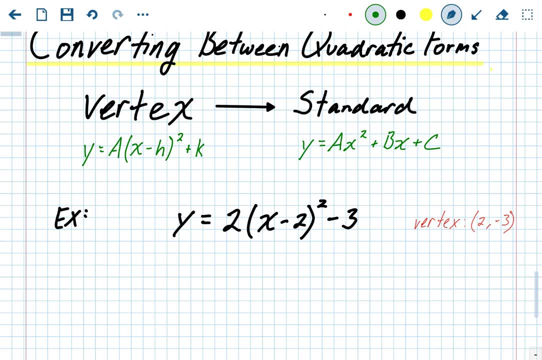 Okay, always good to figure out what you know, All right, so now let's convert it. Let's put it from vertex form into standard form. The steps for this. the first thing you're going to have to do is expand. Okay, so what the expand means is, instead of writing, x minus 2 squared. 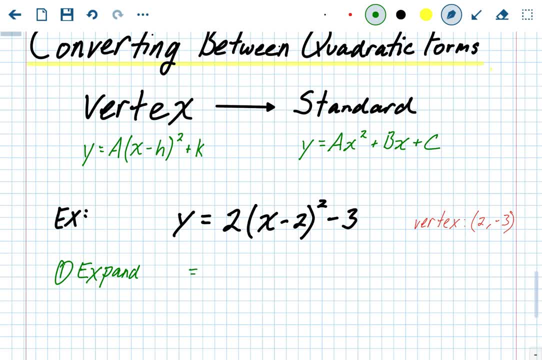 we're going to expand that out into two binomials. So the 2 out front, the a value, is 2.. So again, our a value at the end should be 2.. So we're going to expand that out into two binomials as well. 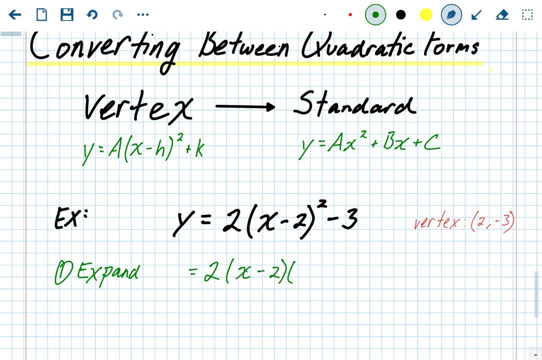 And, like I said, instead of doing x minus 2 squared, we're going to rewrite it as x minus 2 times x minus 2.. So remember, x minus 2 squared just means x minus 2 times x minus 2..